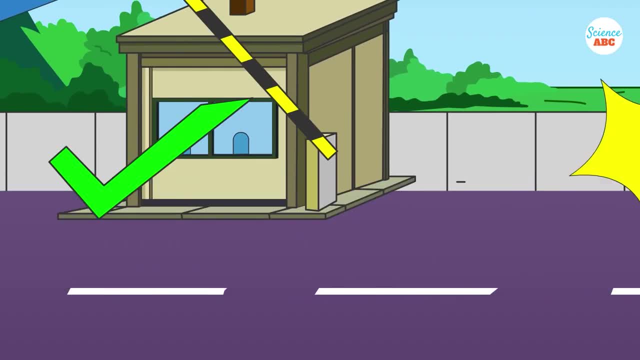 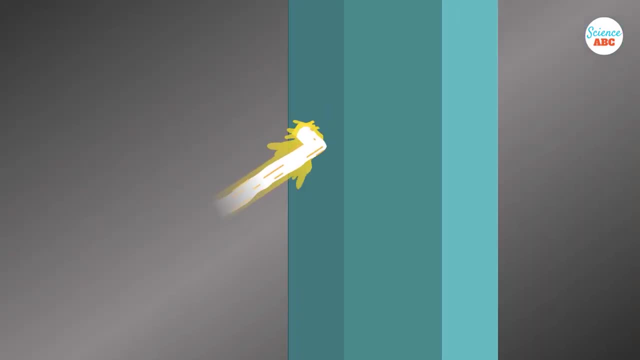 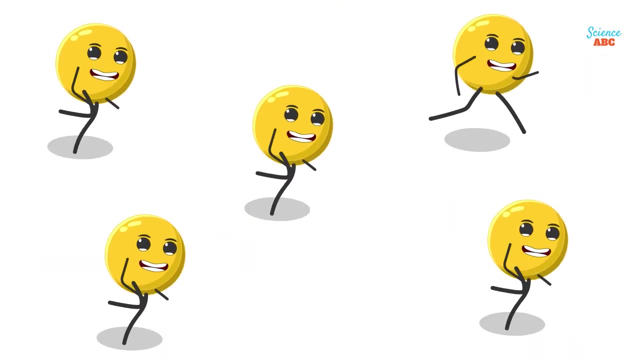 granted passage if you pay the required toll amount. The photoelectric effect works in a similar way. When light, a type of electromagnetic radiation, falls on the surface of a metal, it ejects electrons from the surface. This happens because light is made of massless particles, called 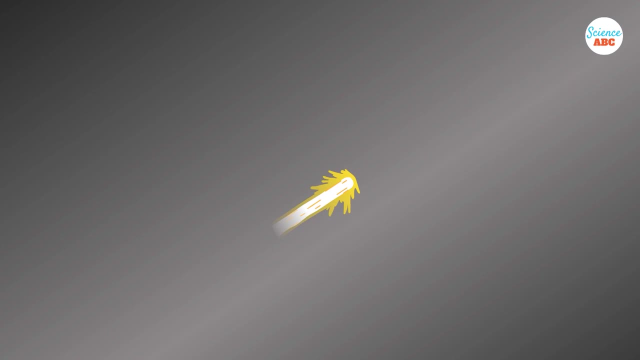 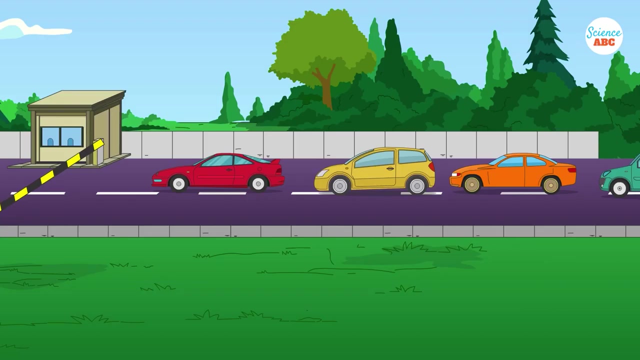 photons which possess a certain amount of energy. When these photons strike the surface, they knock electrons off the surface. When these photons strike the surface, they knock electrons off the surface. We call these photoelectrons. In our toll booth example, the approaching cars represent 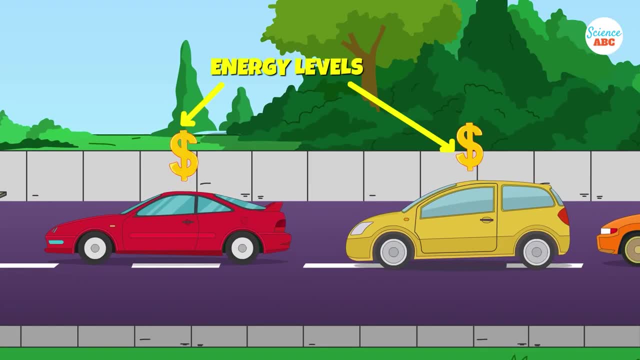 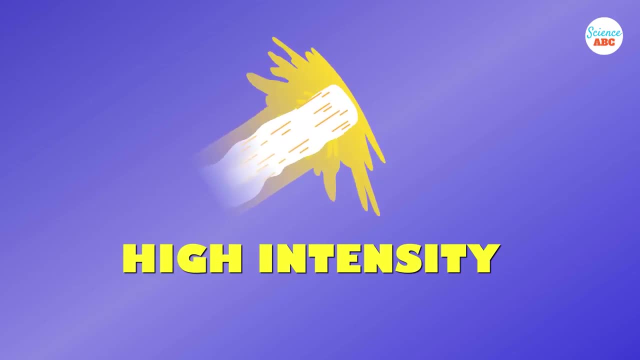 photons. their money represents the energy levels of photons and the act of passing through the toll booth represents the photoelectric effect. You'd think that if a bright light, or in technical words a high-intensity light, is directed at a metal surface, it would knock off quite a few. 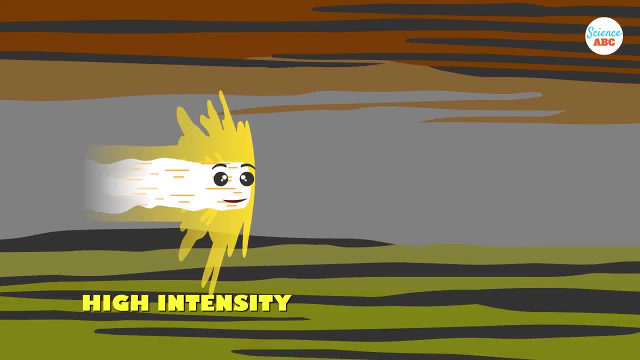 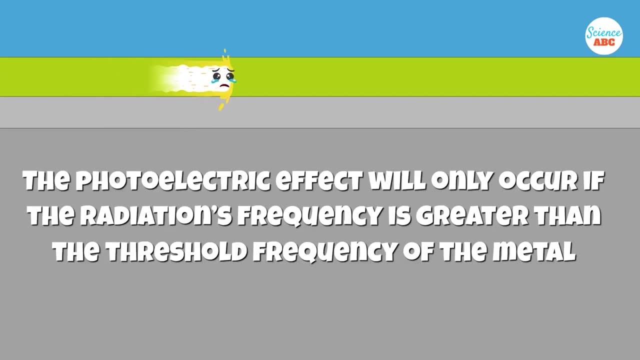 electrons right, Not always. Just because a light ray has a high intensity doesn't mean that it will cause the photoelectric effect. It can only happen if the frequency of the light rays is equal to or greater than a given value known as the threshold frequency of the metal. Look at this graph. You can. 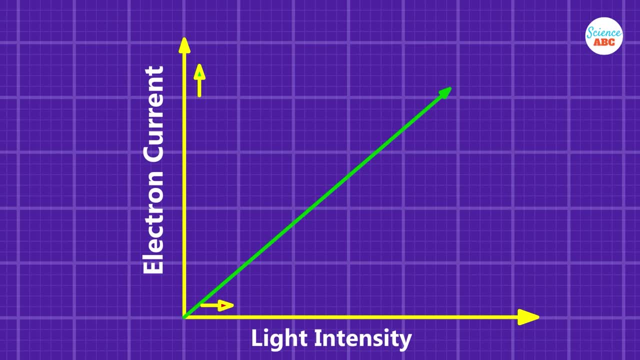 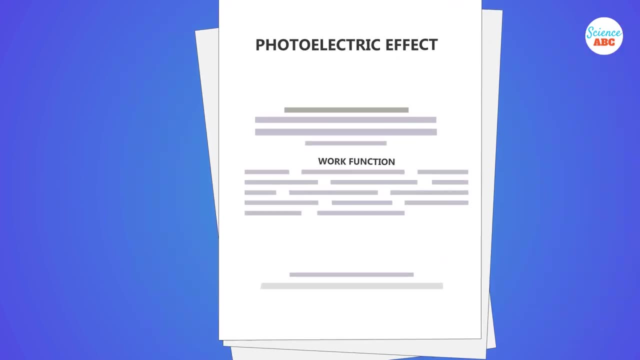 see that the number of photoelectrons emitted increases as the intensity of the incident light increases. When learning about the photoelectric effect, you'll often come across the term work function. This refers to the minimum amount of energy needed to remove an electron from a metal. 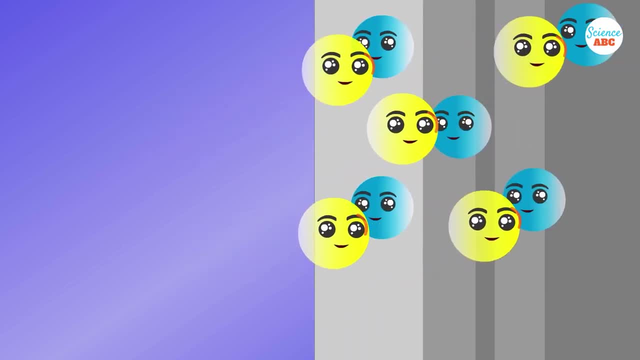 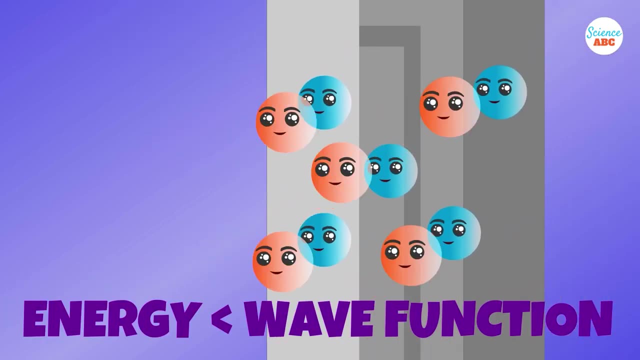 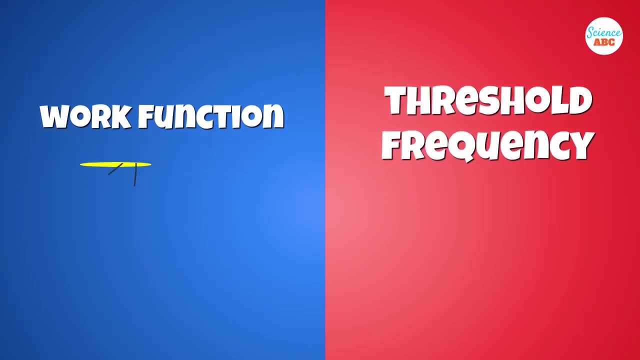 surface. If photons with enough energy hit the surface, they can transfer their energy to the electrons, allowing them to escape. If the energy of the incident photons is less than the work function, no electrons will be emitted, regardless of the intensity of the light. As you can imagine, 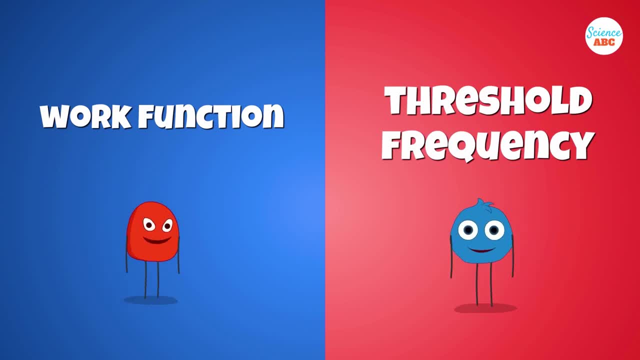 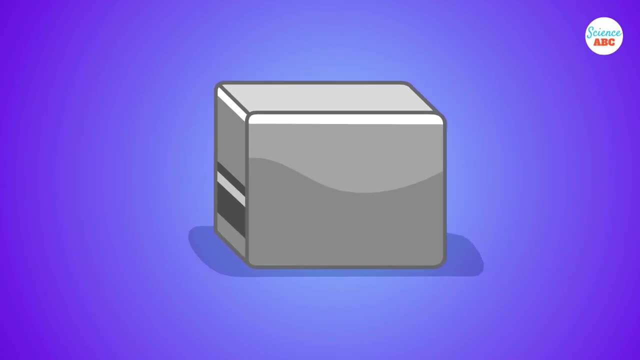 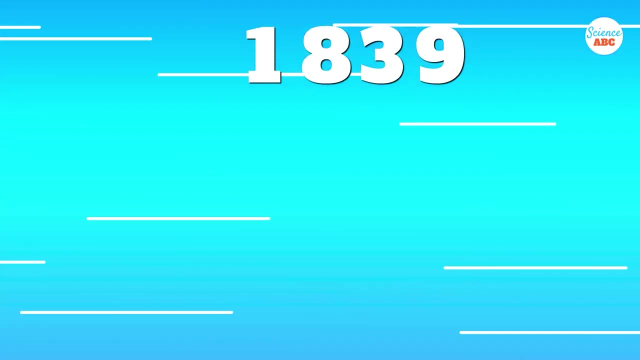 work function and threshold frequency are closely related. Mathematically, the work function equals the product of Planck's constant and the threshold frequency. In simple words, if you know the value of an electron's threshold frequency, you can determine its work function. In 1839, French. 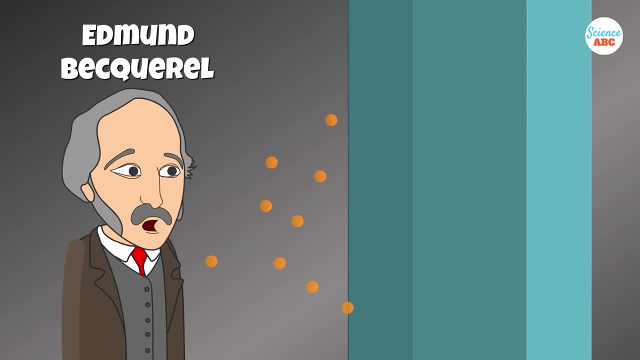 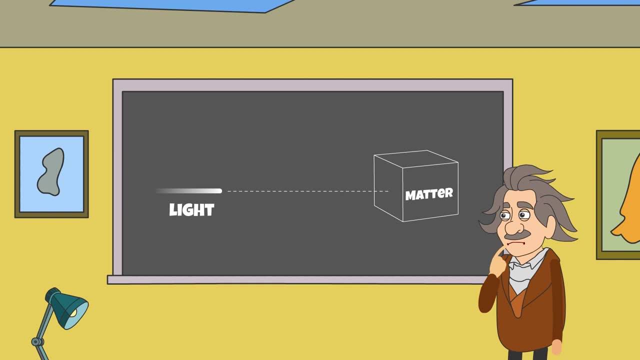 physicist Edmund Becquerel first observed the photoelectric effect. Later, in 1905, renowned scientist Albert Einstein described the interaction between light and matter, revolutionizing our understanding of light. For his work, Einstein was awarded the Nobel Prize in Physics.